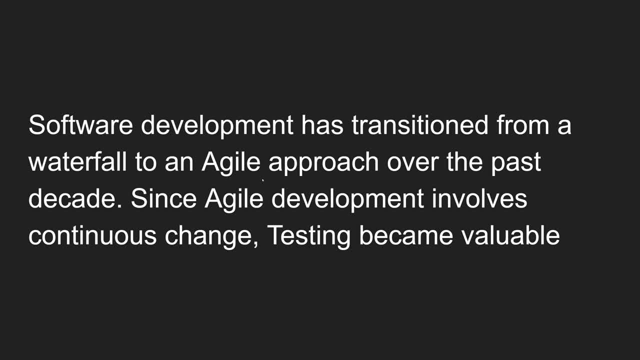 The different possibilities that are given And the security systems or devices are detailed. place the thing down here. gör the top screen. now, when you click on the top screen, guys, you get. lets go to the software Videos for testing Software которu has shown. 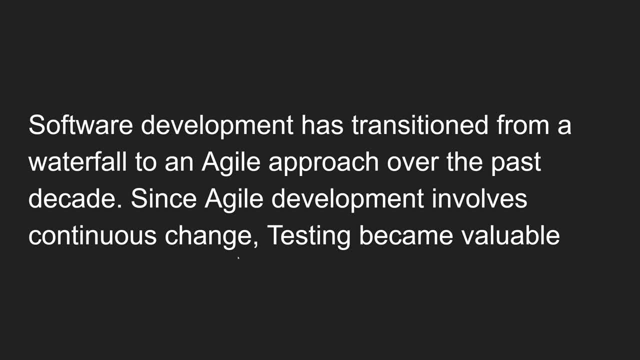 Default modelhehe, So for testing Pow. So you will be having a sprint and you will be having lot of tasks in that sprint and we will need to complete those, all the tasks in that sprint, so that at the end the sprint will be closed. 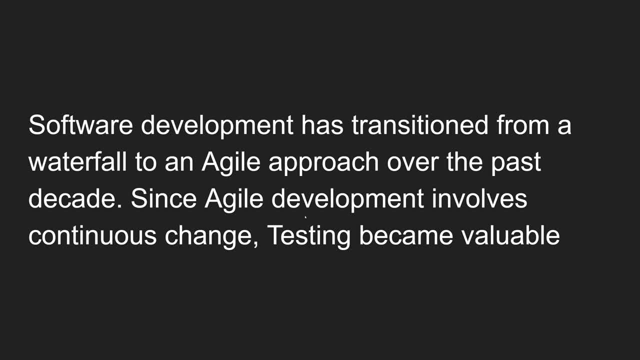 So now in this agile development, what we will be having: we will be having so lot of continuous changes, so we will be developing a lot of continuous changes. So in this agile development approach- so we will- we need testing becomes more valuable. So testing is the main foundation of this agile development. why? because lot of changes. 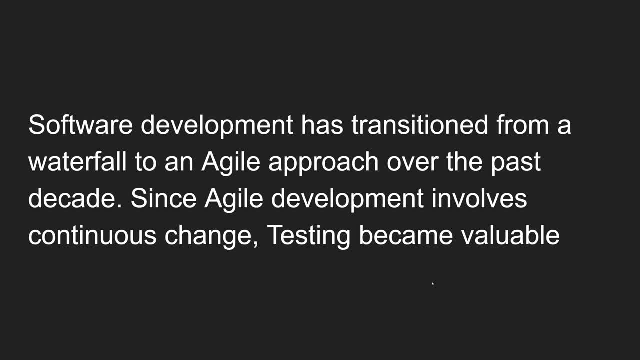 we will be doing in this agile development, and that rigorous testing is needed for this one to, in order to have a continuous development, So in order to have our application to be able to have bugs free. So we need the testing, as well as testing also in the parallel. 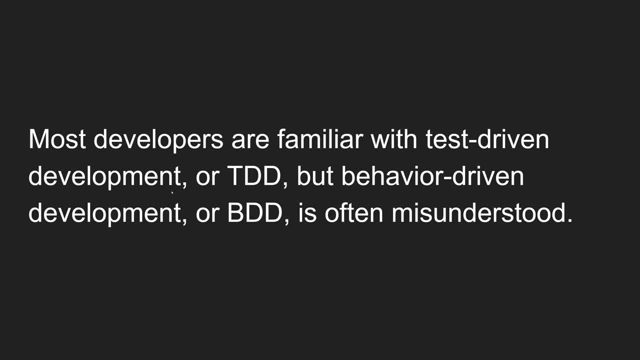 So most developers are familiar with that test driven development. So it was developed in around 1999 or something like that in the 2000s. So most developers are familiar with the test driven development. So why? Because lot of Articles or documentations available in the internet market. 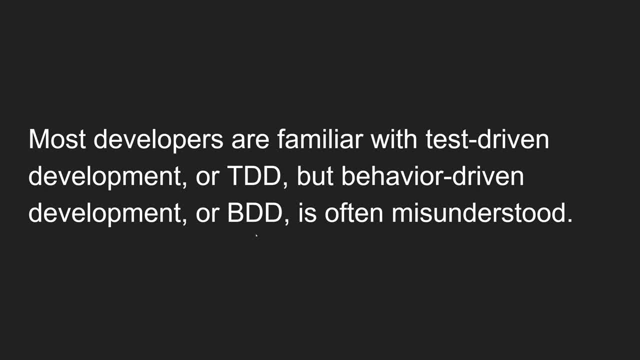 But behavior driven development, or BDD, is often misunderstood. So why? Because this behavior driven development is somewhat misunderstood. So why? Because test driven development is long time available in the market. So most of the developers who are working right now so they know about this test driven. 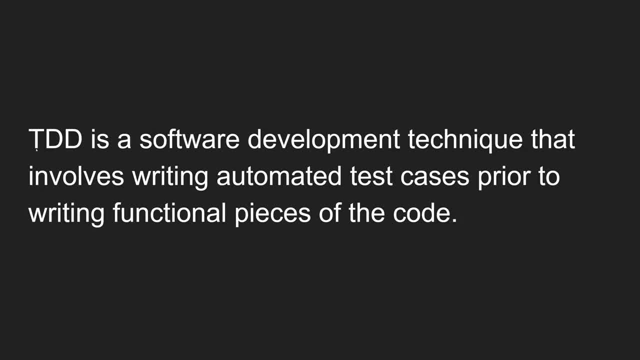 development. So TDD. now let's try to learn about this TDD. What is this actually TDD is? TDD is a software development technique that involves writing automata Test cases prior to writing functional pieces of the code. So here this is the definition, actual definition. 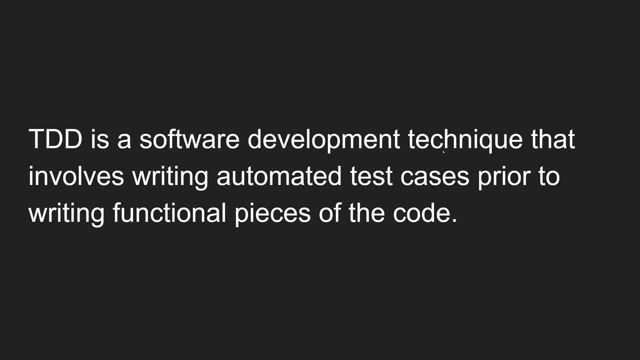 So what is this one is TDD? is a software development technique or a practice, whatever it may be. So that involves writing the automated test cases. So that means so first before writing any piece of code. So if you have a logic to be implemented before implementing that logic, first you will write. 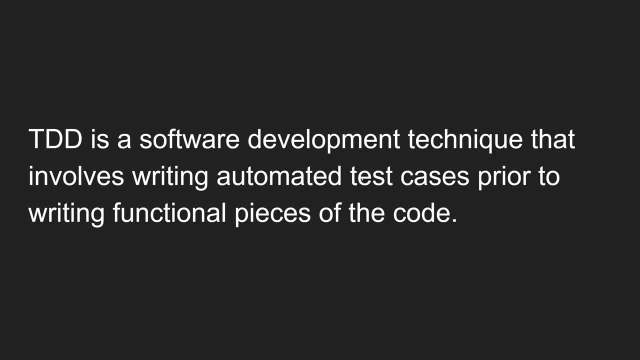 the test case for that logic And now you will try to run the test case And you will get the test case fail. Why? Because you didn't not yet implemented the logic for the test case. Now you will write, you will try to implement that logic. 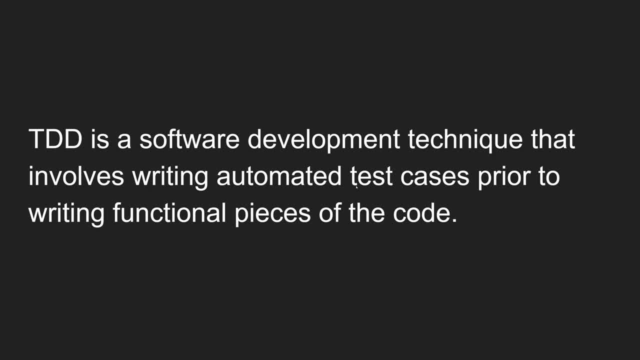 So now you will make that test case pass. So this is the test driven development. So the name itself indicate that test will drive your development. So the test cases drives your development. So that means if any logic you want to implement is you first, you will write the test case. 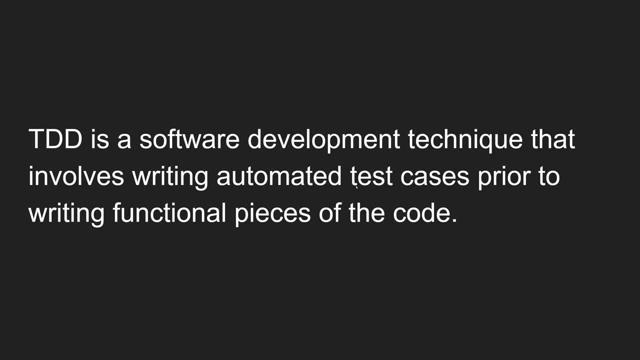 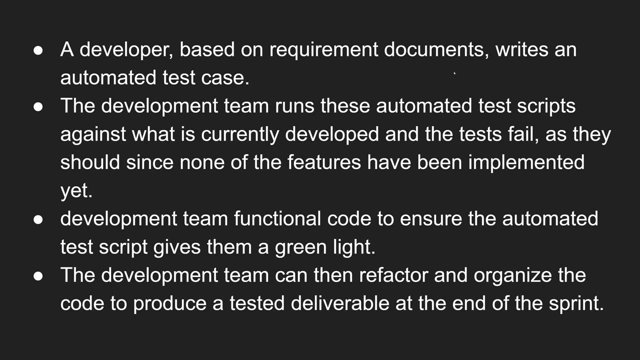 for that logic and you will try to make the test case pass. So by writing that logic. So this is the process how the test driven development will undergo. So first, a developer: based on the required documents, he will write an automated test case So he knows he will get the requirement document. and by taking this requirement document, 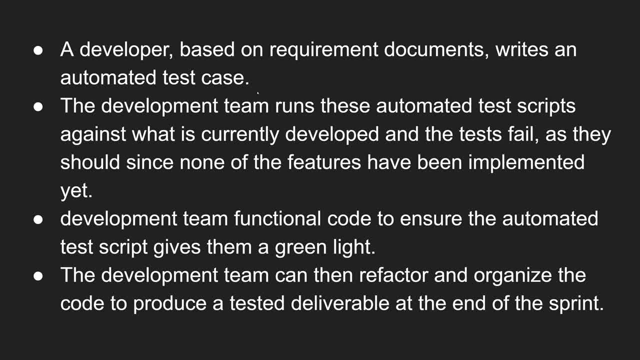 So he will write a test case. So he will not write the logic First, he will write the test case. So the development team runs this test scripts. So, whatever the test cases, we have got it, So we will. we will run this test cases. 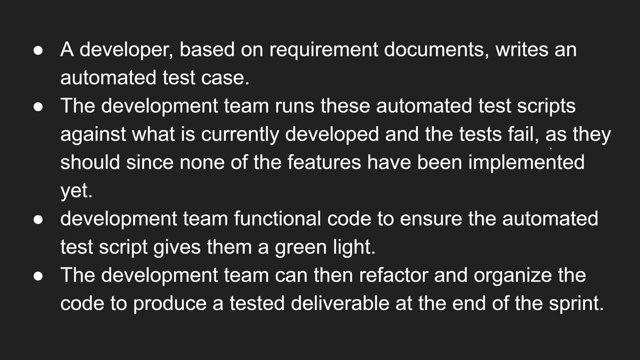 Now what will happen? So we will get this all: test fail. Why? Because so none of the logic has been implemented. Those requirements has not yet been implemented. So only the test cases are implemented, So as they should. none of the features have been implemented. 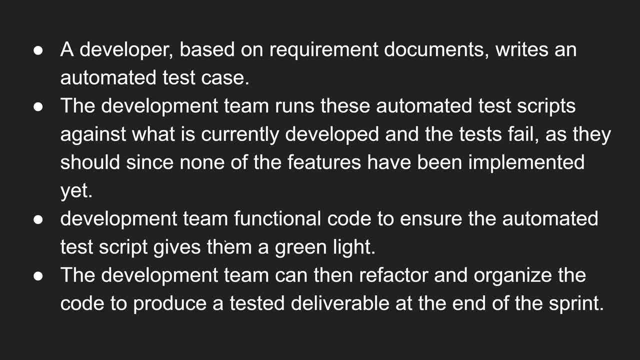 Now the development team. what it will try to do is the development team try to implement those functions making those test cases pass. So now they will implement this functional code to ensure that automated test cases should pass. should green light? green light means it should pass. 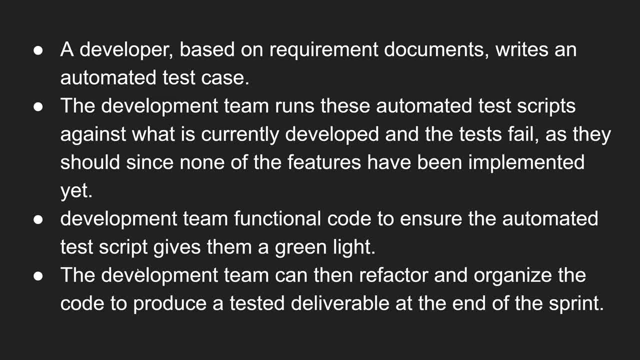 Now. so, after making all the test cases pass, now the logic has been implemented, Now they, what they will try to do is the development team will try to refactor the code. So, if they possible, they will try to refactor the code, what they have implemented. 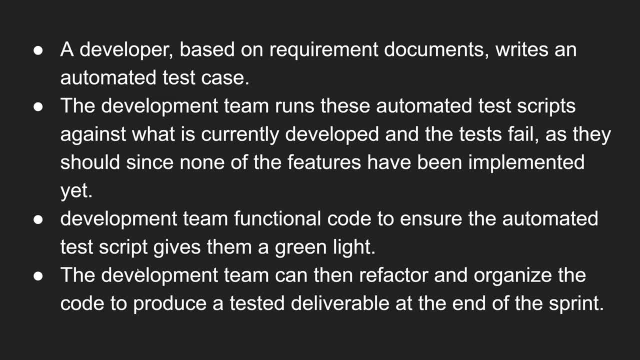 And again, they will try to run the test cases so that the logic, the refactor code, what they have did, it also has to get passed. So this is the process, what they will be trying to do. So, whatever the logic or whatever the requirement, they got it. 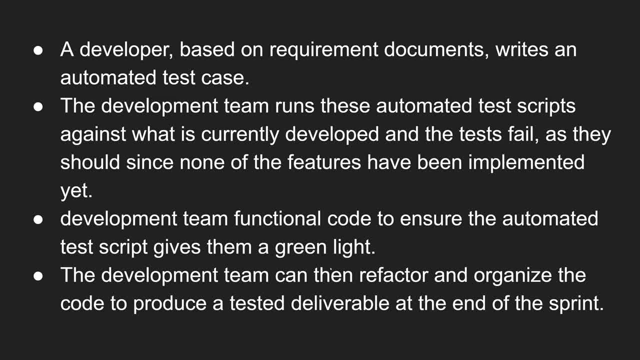 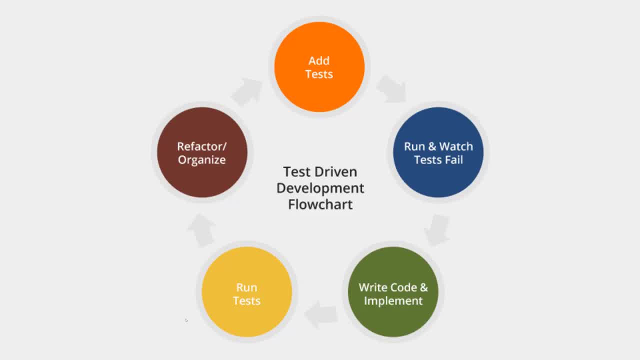 So first they will write the test cases for that logic and now, after implementing the test cases, they will write the logic according to the test case. So this is the test driven development. So pictorial representation of this test driven development will be looking like this: 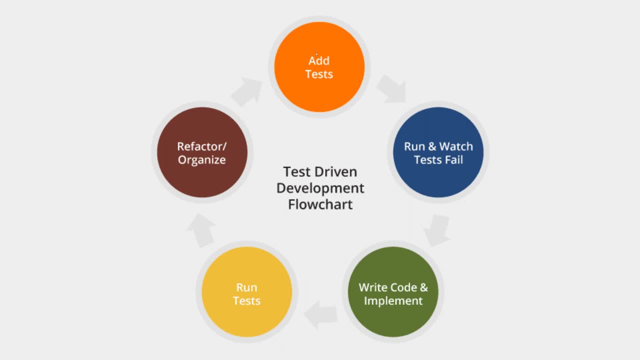 So first we will try to add a test, So after getting the logic, we will try to, So we will add the test, and after adding the test, we will run and watch. So now, automatically the test will fail. why? because the logic is not yet present and we 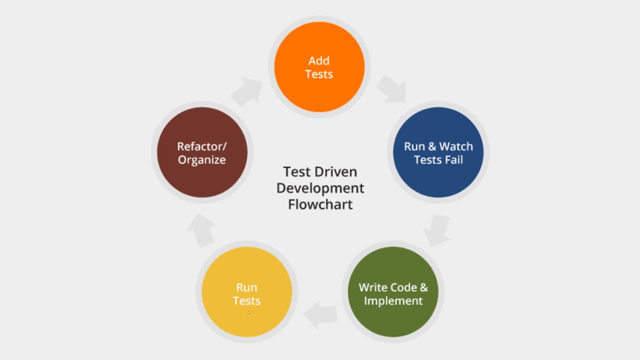 will write the code and we will implement. and again we will run the test. So if it pass means then again we will refactor and organize the code. so, whatever the code we have written, so we have to make the test pass now we will refactor, we will organize. 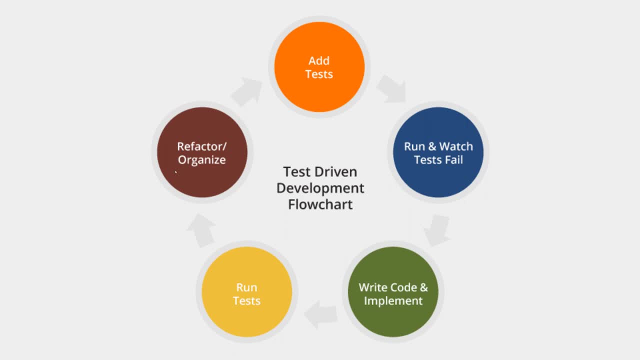 the code and again we will try to run the test. if all the test pass means ok, fine. if any of the test fail means again we will try to make the test. we will try to change the code to make the test pass. Again, the same process repeats. 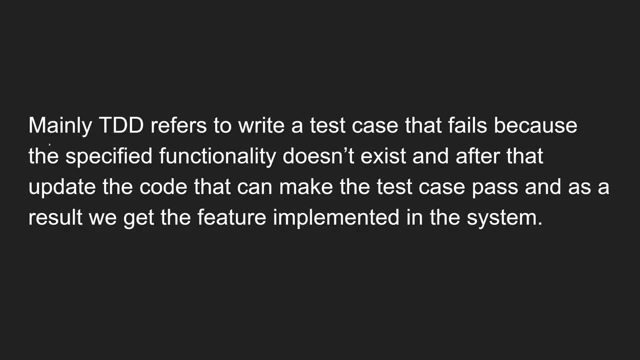 So this is the test driven development flowchart. Ok, mainly TDD refers to write a test case that fails. so what the TDD? what we have learned up to know? so TDD refers to write a test case that fails because the specified functionality doesn't exist and after that update the code that makes the test case pass and, as a result, 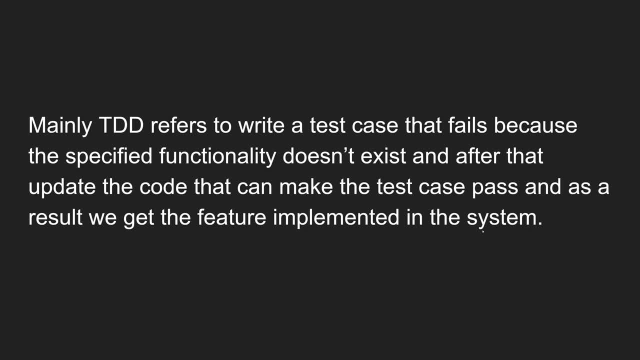 we get the feature implemented in the system. so in this way, the pieces of code, so we will write the test case and we will make the test case pass and these all the pieces of code combinedly will make the features. so this is the test driven development. so, if you want, 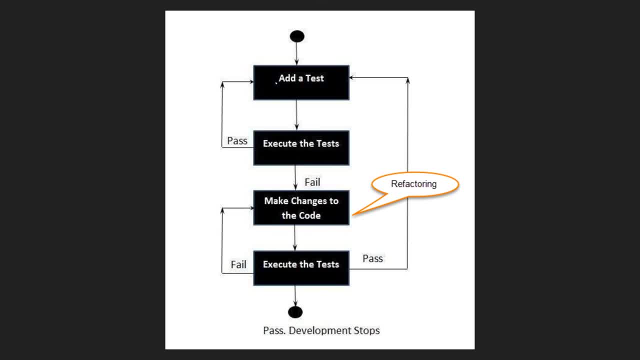 to see the flowchart also. this is also one type of flowchart. so what is this one? add a test case. so same thing. execute the test. so if it pass means again you will write the add another test. if it fails, means make changes to the code. so if the code is not present, 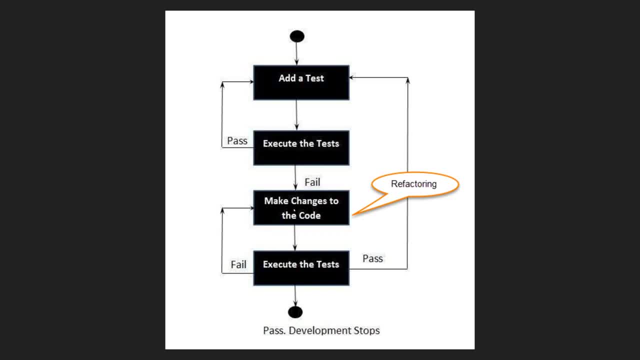 means you will write the new code and all those things and if you want, you can also refactor the code here and again. executes the test if anything passed, means you can also add a test again, new test or other way. fail means you also make it changes to the.